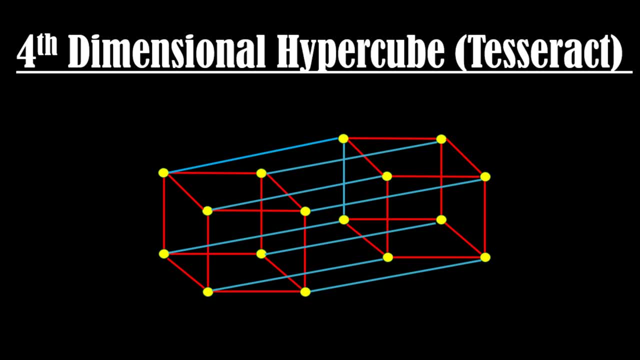 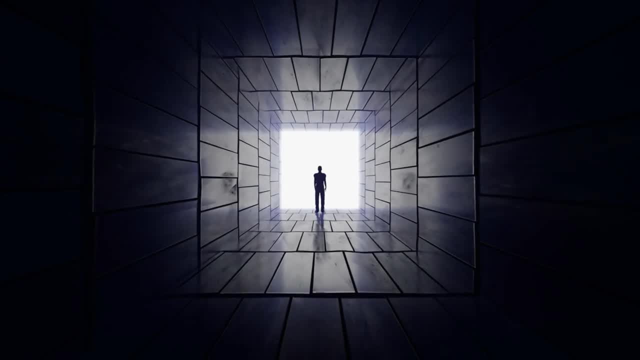 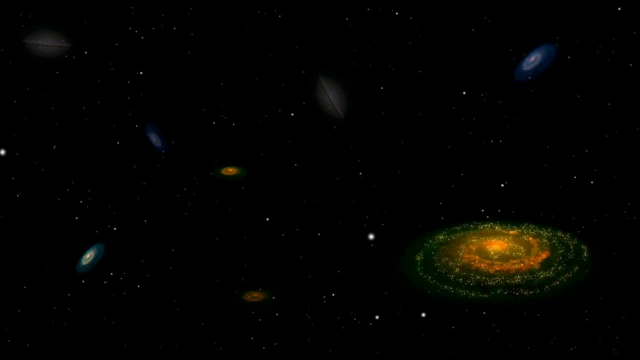 point of view, then, hypercube is a 4-dimensional object, also called a tesseract, 5th dimension. A 5th dimensional being can move either in the past or in the future, and even at different locations at the same time. Actually, parallel universes exist in this dimension, So you may. 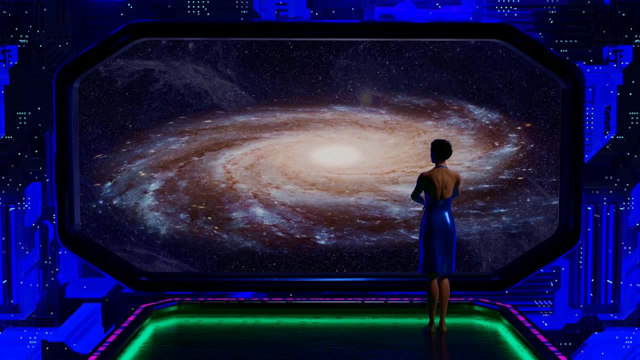 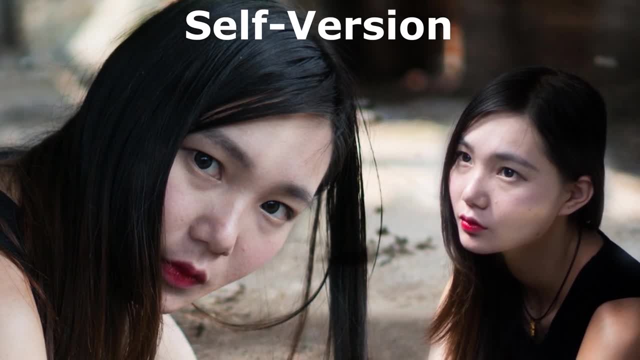 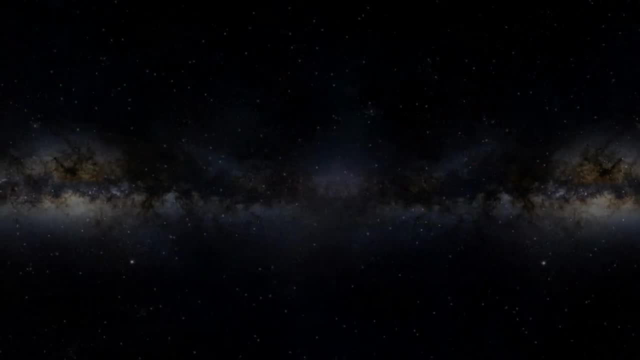 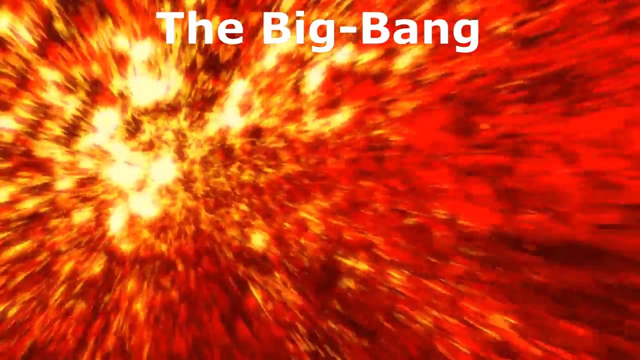 5th dimension is that you cannot meet your self-version directly using shortcuts to another timeline of parallel universe. 6th dimension: In the 6th dimension, all the parallel universes must have the same beginning, that is, the Big Bang. A 6th dimensional being can see all the presents. 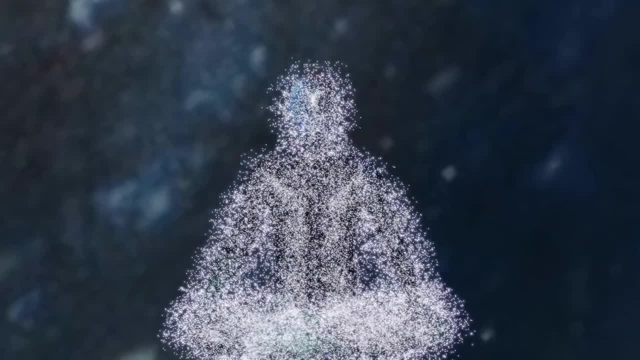 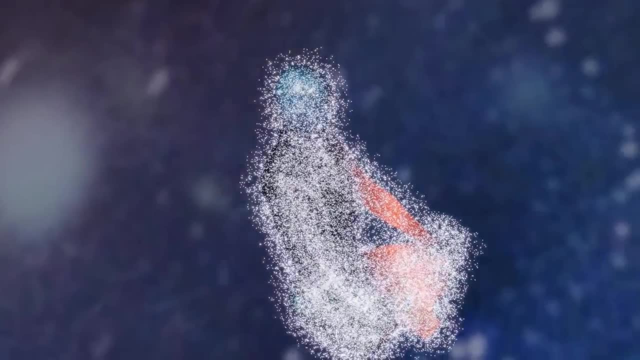 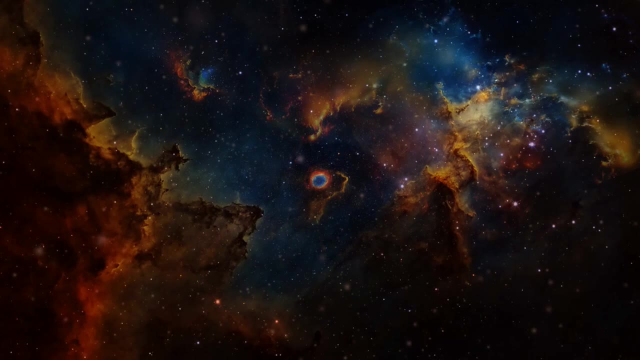 pasts and futures of all the parallel universes. In this dimension you can easily jump from the timeline of your universe to any point present on the timeline of any parallel universe, which was impossible in the 5th dimension, 7th dimension. 7th dimension can have infinite. 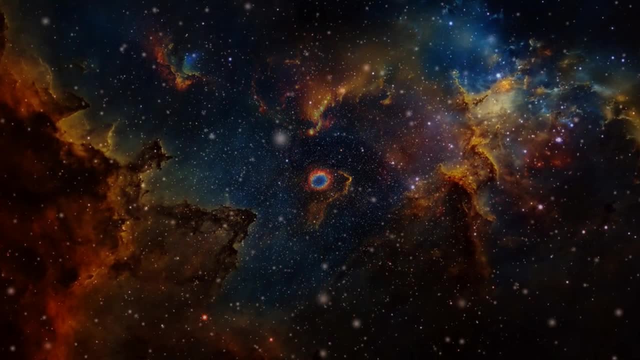 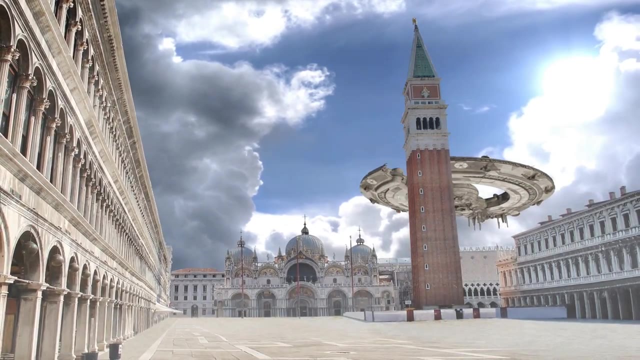 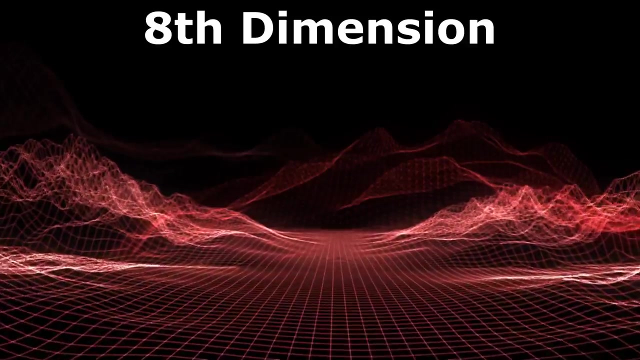 number of universes. These universes may have originated from different start conditions, not just the Big Bang. A 7th dimensional being can have infinite forms of itself and can move from one universe to any other universe. 8th dimension- The 8th dimension has a plane of all the possible presents. 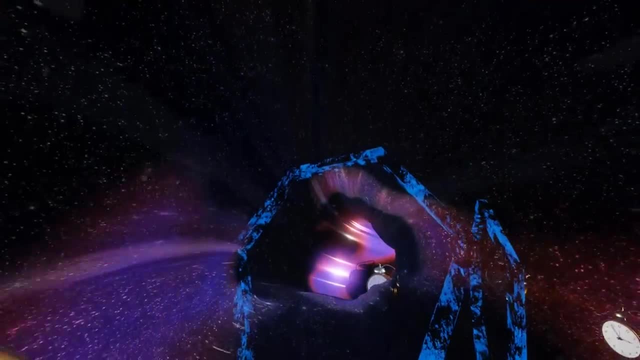 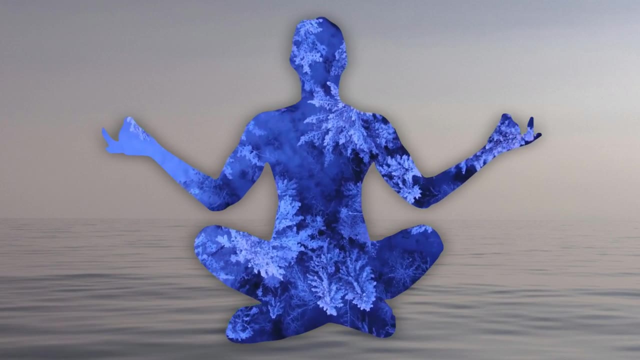 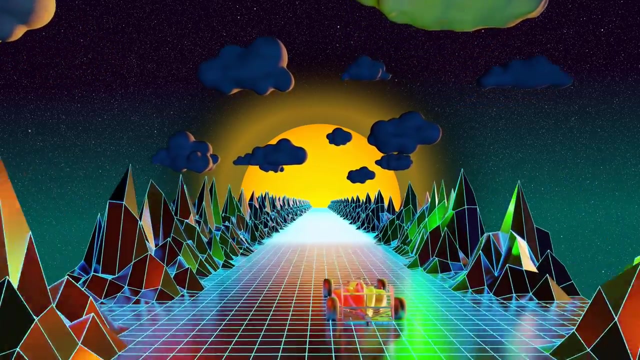 pasts and futures, for all the infinite number of parallel universes. And all these infinite universes extend up to infinity. String theory says in the 8th dimension objects do not have any physical existence. They can change shape, size and appear or disappear instantly. So it may be somewhat similar to the virtual reality. 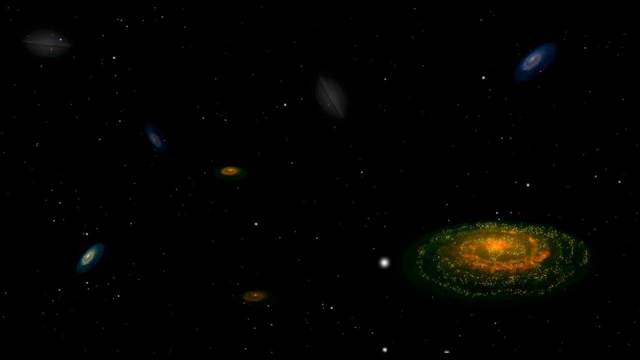 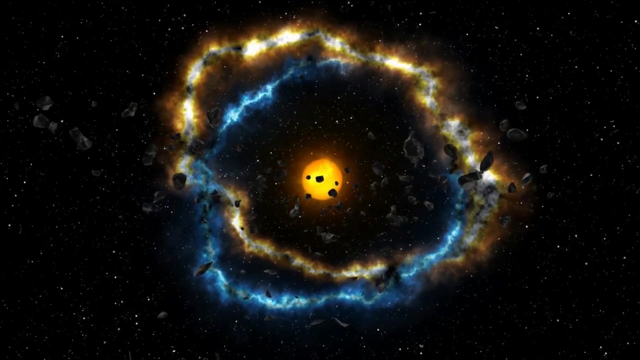 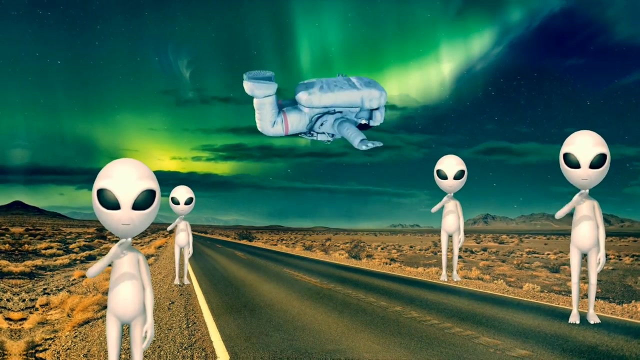 9th dimension. Infinite number of universes exist in the 9th dimension that may have their own laws of physics, separate conditions and probabilities of their origin. Surprisingly, in the 9th dimension, many civilizations or aliens may coexist at the same place without